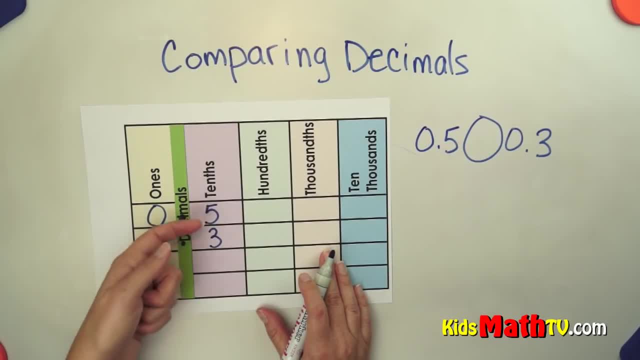 the ones first. The ones are zero. so that doesn't help me. So I go to my tenths. So I have five tenths or three tenths. In this case, five tenths is more than three tenths. You can think of this as money as well, if you put a zero here. 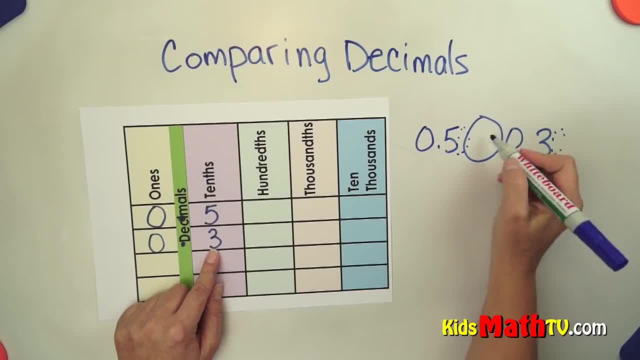 This would be fifty cents and thirty cents. I'd rather have fifty cents than thirty cents. So five tenths is greater than three tenths. And remember: the big open mouth goes towards the bigger number. the small dot or the small point goes towards the smaller. 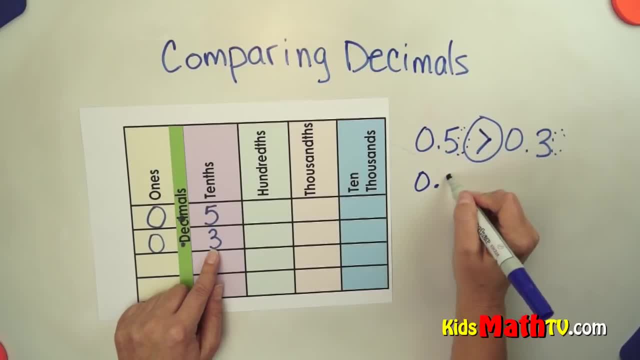 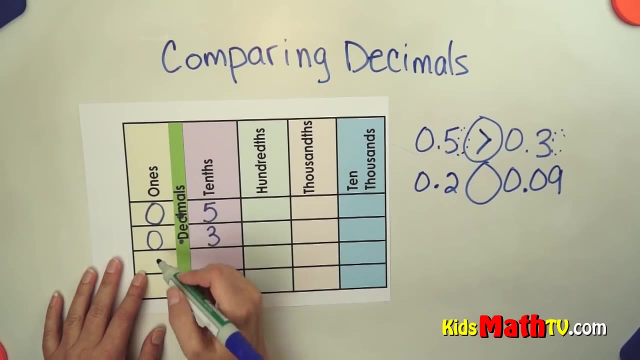 number. Let's try another one. How about zero and two tenths, compared to zero and nine hundredths? Many people see this and go: oh, that one's bigger, Nine is bigger than two. Well, let's put it on the, on the on the decimal chart here. So we 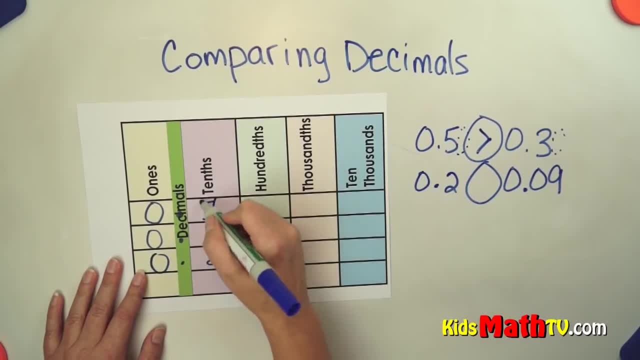 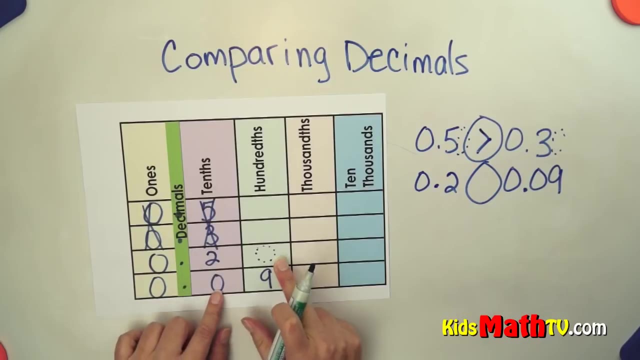 have zero and two tenths- I'm going to cross these out, so I don't look at them- And we have zero and nine hundredths. Okay, this is more like 20.. This is 20 hundredths, or like 20 cents. This, however. 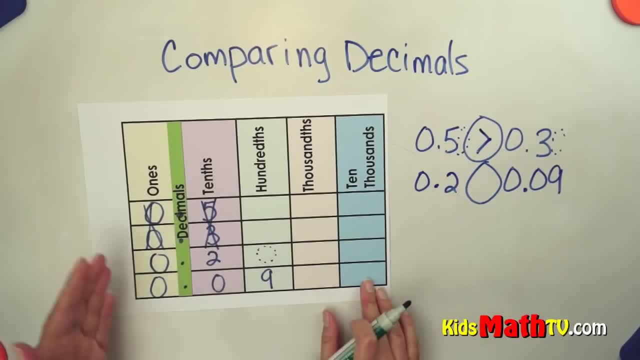 is only nine cents. It's nine in the hundredths place. So if we look, 20 is actually larger than nine. 20 hundredths is larger than nine hundredths because it has two tenths and nine hundredths has zero tenths. So two tenths is actually greater than nine hundredths because there are two tenths. 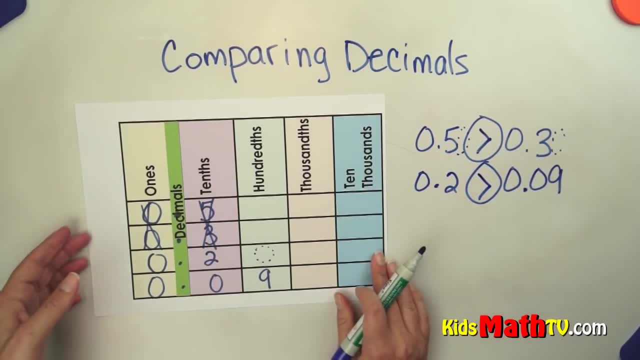 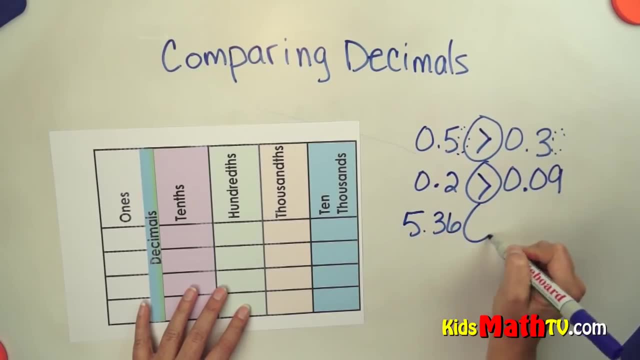 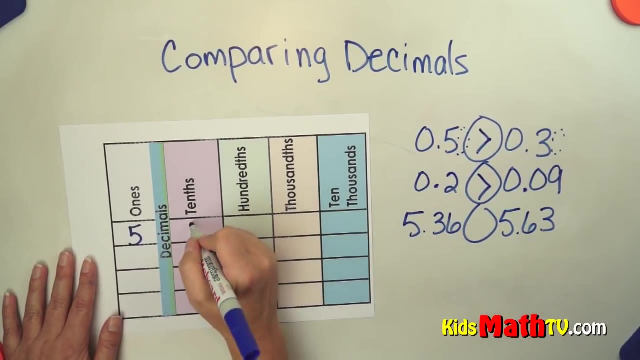 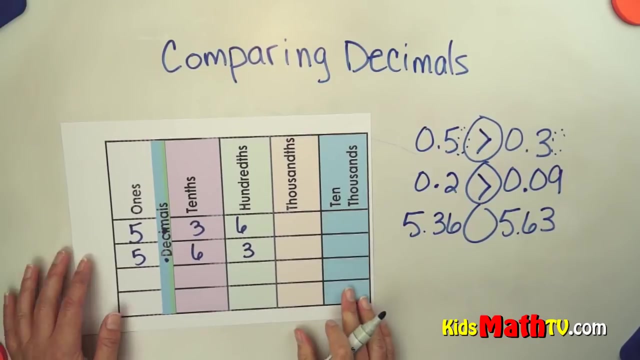 in two tenths and zero tenths in nine hundredths. Let's try a couple more. How about five and thirty six hundredths compared to five and sixty three hundredths? So we put the ones down first. Decimal thirty six hundredths, Five and sixty three hundredths, So the ones are. 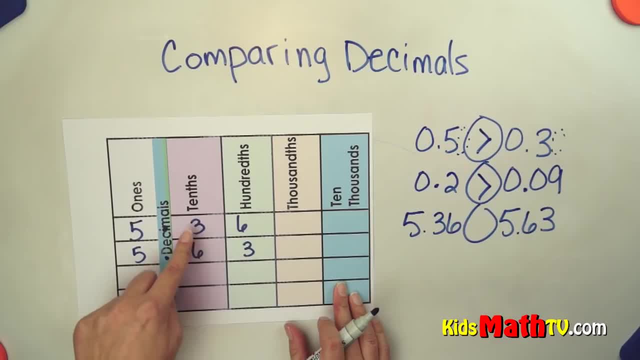 the same. That doesn't help us any. We're going to go to the tenths place. The tenths place, This is three tenths and this is six tenths. So this is really as far as we need to look: Six tenths.